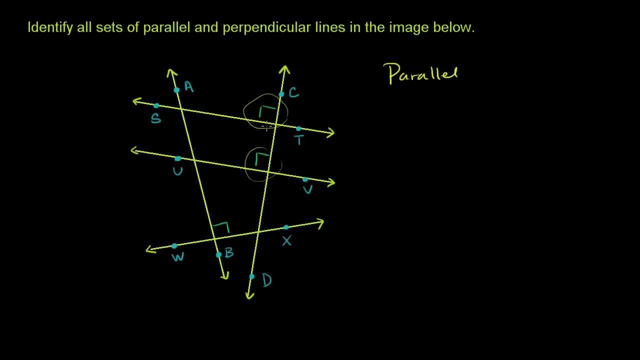 they both intersect line CD at the exact same angle, at this angle right here, And in particular it's at a right angle. And if you have two lines that intersect, a third line at the same angle. so these are actually called corresponding angles and they're the same. 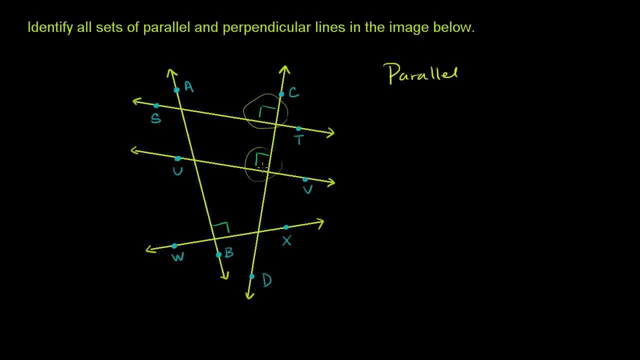 If you have two of these corresponding angles the same, then these two lines are parallel. So line ST is parallel to line UV And we can write it like this: Line ST. we put the arrows on each end of that top bar to say that this is a line, not just a line segment. 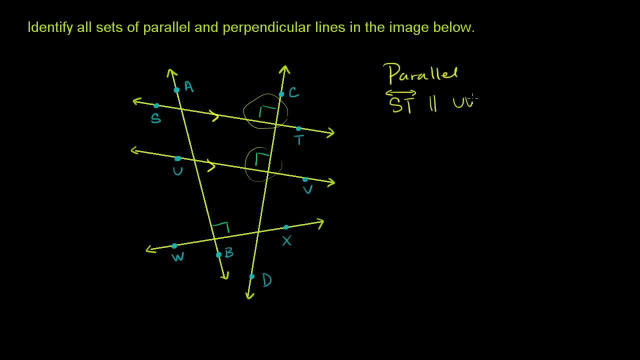 Line ST is parallel to line UV, And I think that's the only set of parallel lines in this diagram. Yep, Now let's think about perpendicular lines. Perpendicular lines are lines that intersect at a 90 degree angle. So, for example, line ST is perpendicular to line CD. 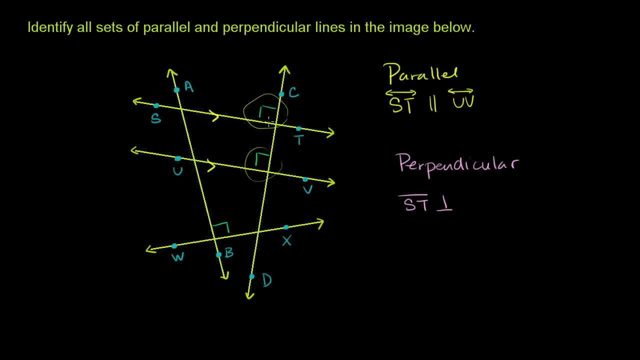 So line ST is perpendicular to line CD And we know that they intersect at a right angle or a 90 degree angle. So I gave us this little box here which literally means that the measure of this angle is 90 degrees. By the exact same argument, line UV is perpendicular to CD. 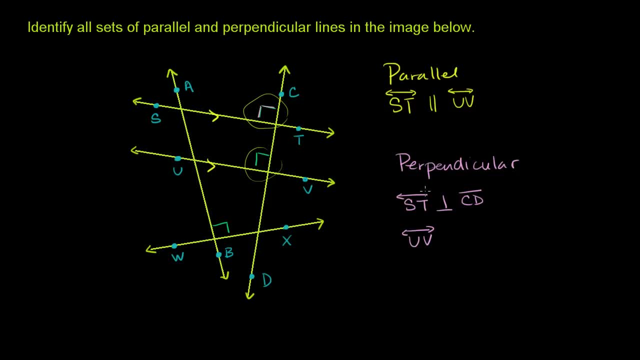 So UV? Let me make sure I specify these as lines. Line UV is perpendicular to CD, So I did UV ST. they're perpendicular to CD. And then, after that, the only other information where they definitely tell us that two lines are intersecting. 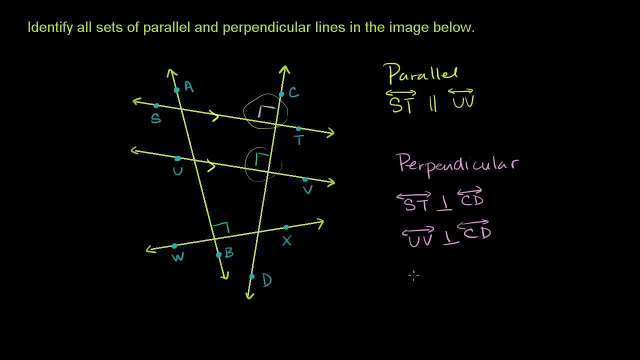 at right angles are line A, So AB is definitely perpendicular to WX, line WX, And I think we are done. And one thing to think about AB and CD: those are definitely not well, they don't even intersect in this diagram. 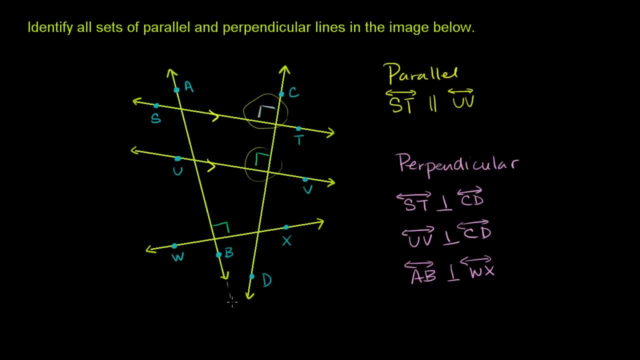 So you can't make any comment about perpendicular, But they're definitely not parallel. You can even imagine that it looks like they're about to intersect And they give us no information that they intersect the same lines at the same angle. So if somehow they told us that this is a right angle, 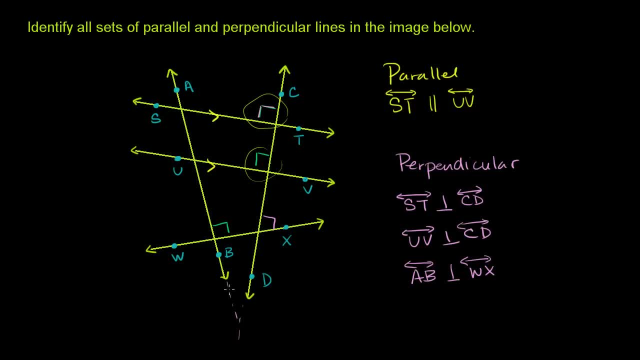 even though it doesn't look anything like a right angle, then we would have to suspend our judgment based on how it actually looks And say, oh, I guess maybe those things are perpendicular. And then, actually, it actually, or maybe these two things.